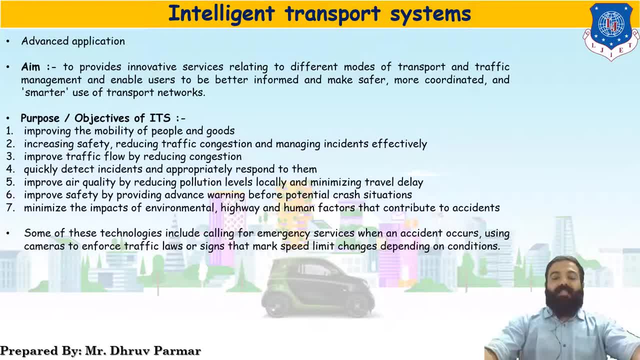 Then Ford quickly detect incident and appropriately respond to that. like in Near about roundabout The accident occurred. So how can you quickly respond, How can you go quickly by this system? then, fifth one: improve air quality by reducing Pollution level locally and minimizing the travel daily. 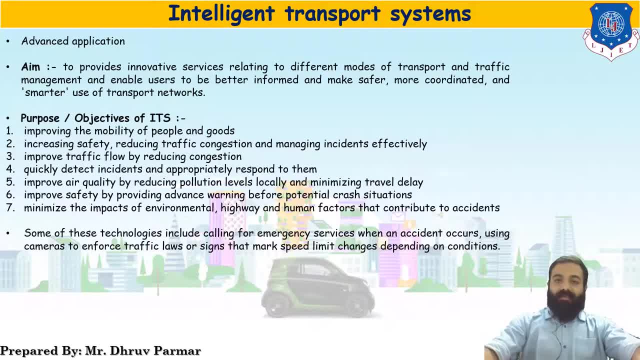 How can you improve air quality so you can use a smart vehicles like based on electrical, based on biofuel, the sequel. improve safety by providing advanced warning before potential crash situation. Some types of vehicle that advanced technology are used to indicate before the accident occur, like the barriers are, or the public's and. 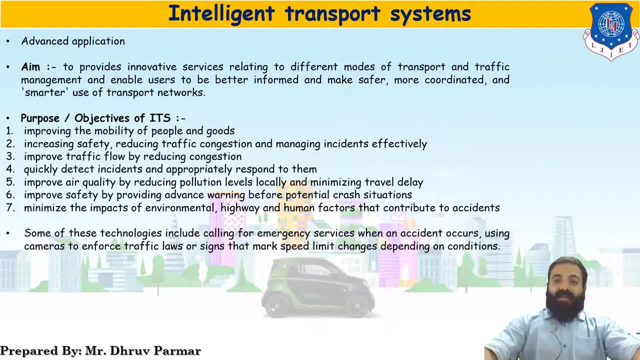 like some obstacles Which are comes Instantly, so that wall To the driver or to people by some advanced technology. then, seventh one, minimize the impact of environmental, Highway and human factors that contribute to X, So that some of the technologies include falling for emergency service when an accident that was using cameras to enforce traffic flow or sign that much speed limit changes, depending on. 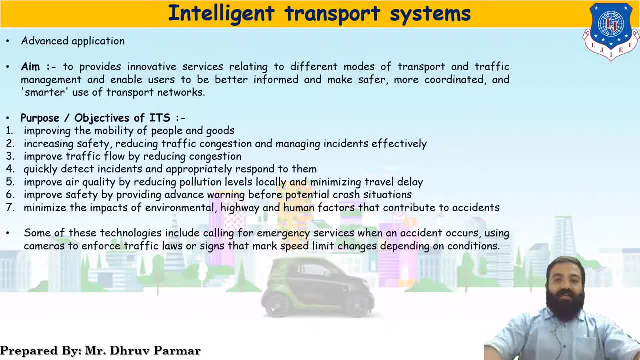 and it all in all, the meaning of the all in all. what is the meaning of intelligent transport is that enhance our facility and our safety by using some advanced technology and reduce the environmental pollution or improve air quality by using different types of fuels which are Renewable. clear, So this, this is the meaning of intelligent transport system. 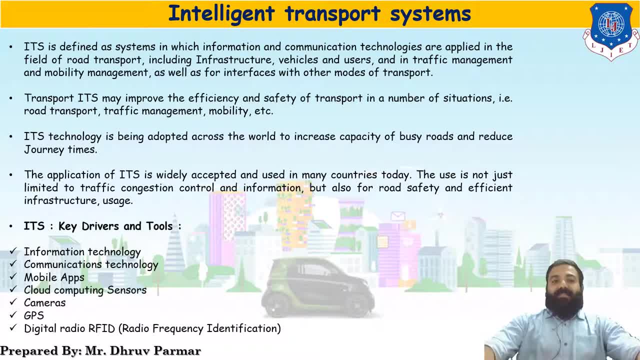 the next one, ITS. ITS is one type of system in which the communication and information technology are applied in the transport system, like including infrastructure, vehicles and user, and in traffic management, as well as mobility management. Transport ideas may improve the efficiency and safety of transport in a number of situations. 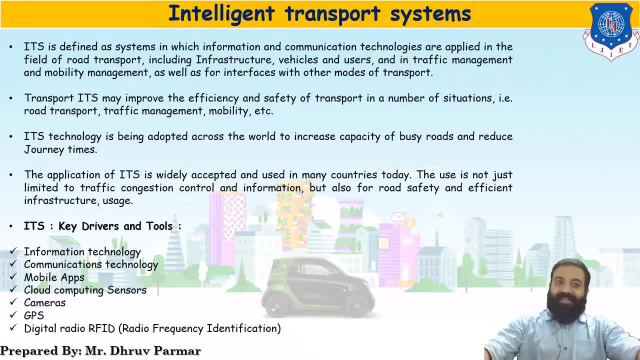 like road transport, traffic management, mobility, As I said that by the using of ITS system, so you can improve or you can reduce the traffic congestion and increase the traffic management and transport system. This system is adopted across the world or throughout the world to increase the capacity. 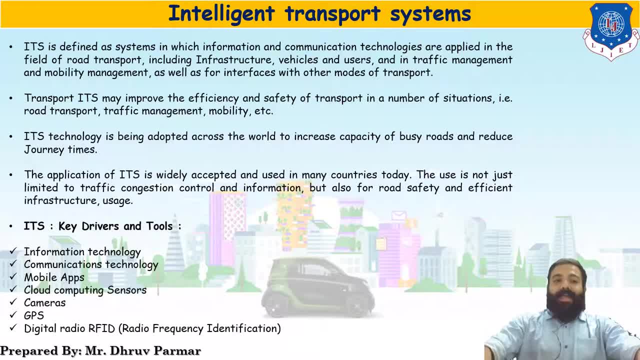 of busy road and reduce journey time. There are widely applications of ITS. So what is ITS? ITS is accepted and used in many countries, like in over India, so the use of not just to limited traffic congestion, but also it improves road safety and efficient infrastructure. 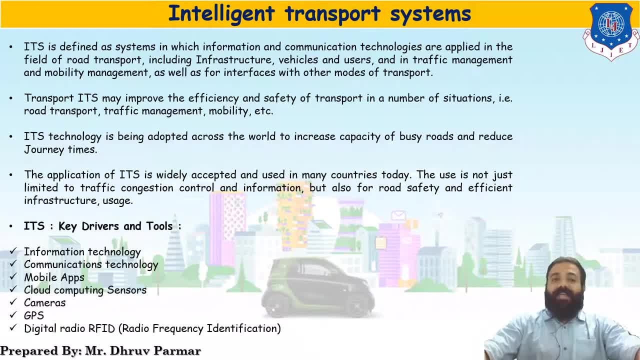 So there are some key tools and drivers which, included in ITS, so like information technology, are used in ITS: communications technology used mobile apps, cloud computing, sensor cameras, GPS, digital radio, RFID. So these drivers and tools which are used in ITS, ITS clear. 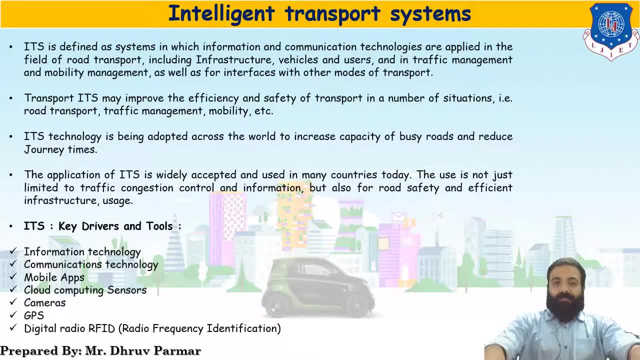 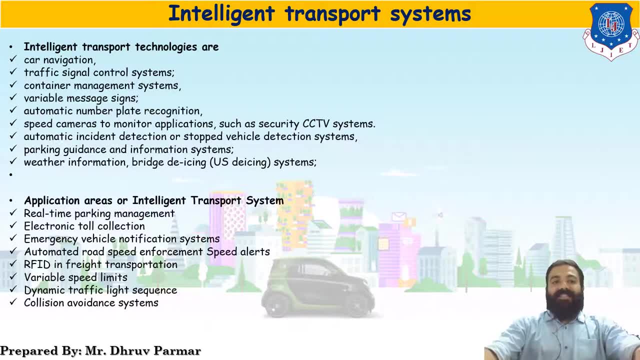 So this is the basic meaning of intelligent transport system. So how can we use the intelligent transport technology? so you can use in car navigation, you can use traffic signal control system and, after, container management system, like in our mudra mudra bot. 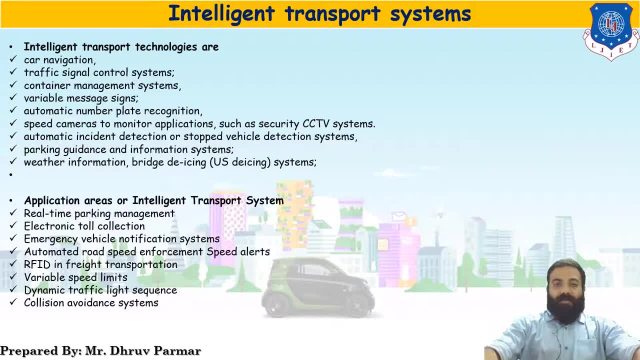 How can manage the particular traffic? How can manage the traffic? How can manage the traffic? So you have to have your big container then and variable message sign so you know that there are different signs of traffic management. clear Then you already about that automatic recognition number plate so you can break the signal. 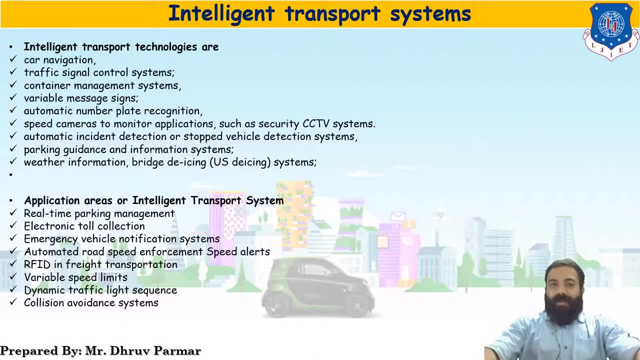 or break the rules so that cameras or that sensor which recognize your number plate and give a file or memo, then speed cameras to monitor applications in the security system, like in out of the India that speed camera used to detect the speed of vehicle and if the speed is higher than the normal speed they find to that 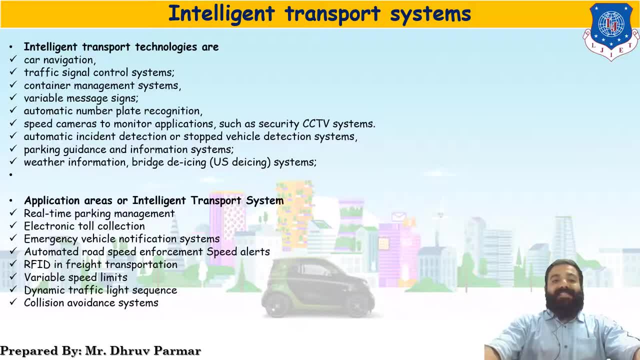 driver. then after automatic incident detection and stop vehicle detection system. like you know that about Tesla clear, so in Tesla you, when the obstacle or any person which comes to the road, so that system or that sensor which warns you that obstacles are near your vehicle, clear parking guidance and information. 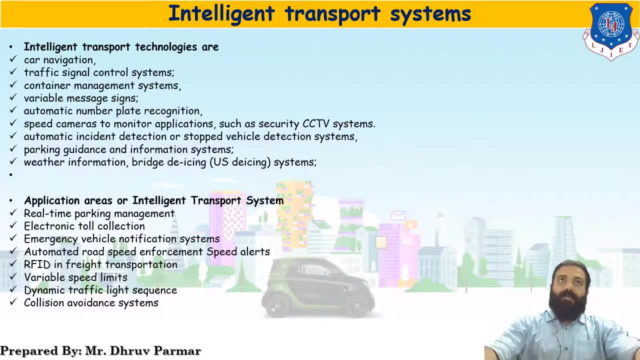 system. like you know that there are automatically parking systems like Aurore and Endeavour or Fortuner, which stop model, then after weather information, with all this using intelligent transport technology. so what are the applications area of intelligent transport system? first one: real-time parking management, electronic toll. 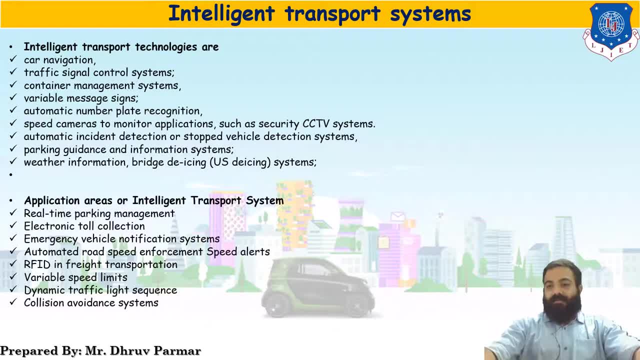 connections like. there are various. there are, as per the Indian government here. so there are barcode, are given collected toll here. if you have not that particular barcode, then you find double amount here. then emergency vehicle notification system, automated road speed enforcement, speed alerts, RFID into freight transportation means. 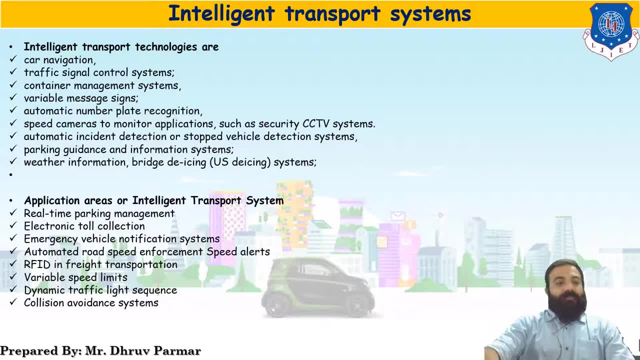 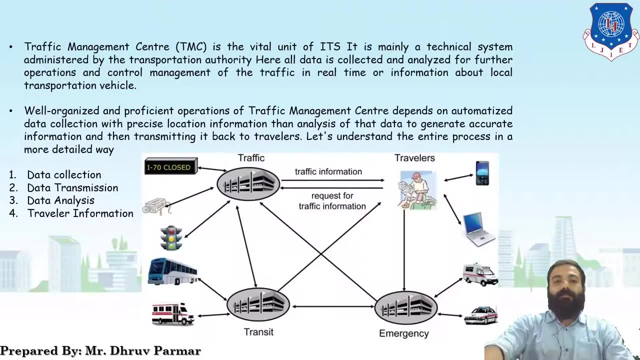 good transportation. variable speed limits, dynamic traffic light sequence, collision avoidance system. these are the use it or applications ofalked. next one: traffic management. traffic management center, that color TMS it is so is the vital unit of ideas, means most important unit of ideas here. so it is. 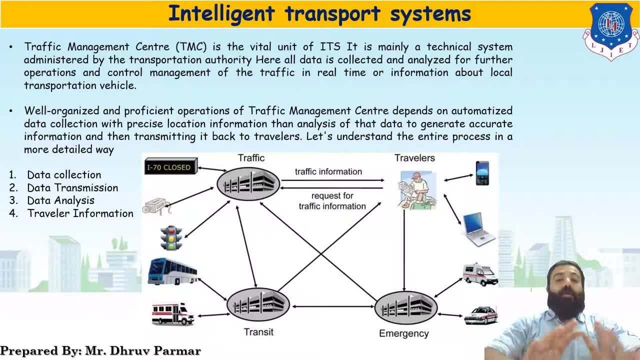 administered by the transportation authority. all data is collected or analyzed for further operations and control: management of the traffic in real time or information about local transportation right now. yeah, the traffic management system is a main important part of, or main important unit of, ideas, because they collect all the data and the admission by 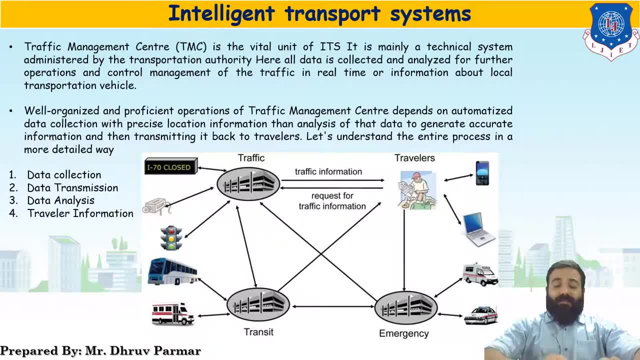 transportation authority and data which will use for traffic management systems and otherwise I can use the some parking design or new road constructions or bridge construction clear, so the plan will be well organized or proficient. operation of EMC depends on automized data collections, which gives local informations and analysis of the data to 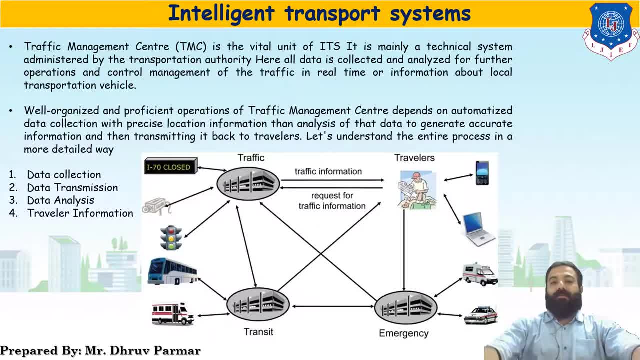 generate accurate information and transmitting to that to travel that process more detail, like a first one. how can you collect? so first that data collection, then data transmission to the EMC- means traffic management center- then data analyzed, then after that data will be get by travel here. so this is a diagram, the data which 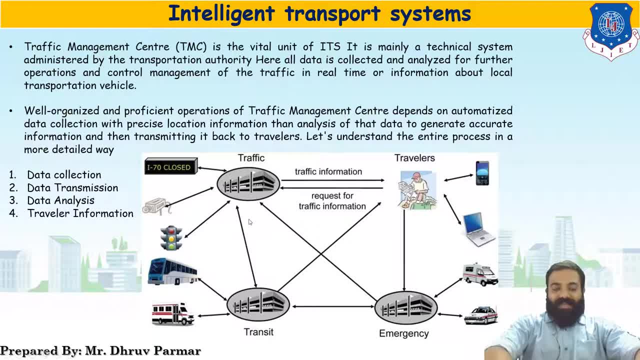 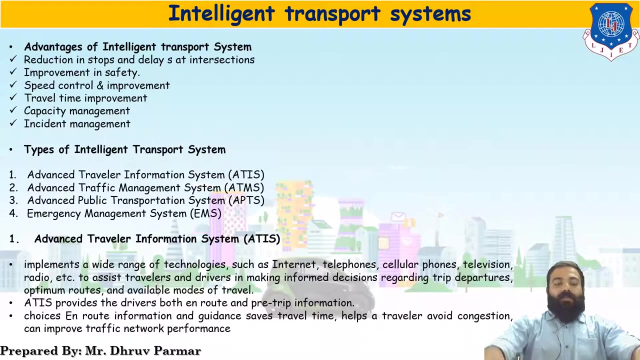 connect to the EMC and by some data collection method clear that transform to data transfer means EMC center and then go to travelers by some mobile applications, by for websites here. so this is a traffic management grilled. the next one: advantages of intelligent transport system. so what are the advantage? the first one: reduction in stops and delays at 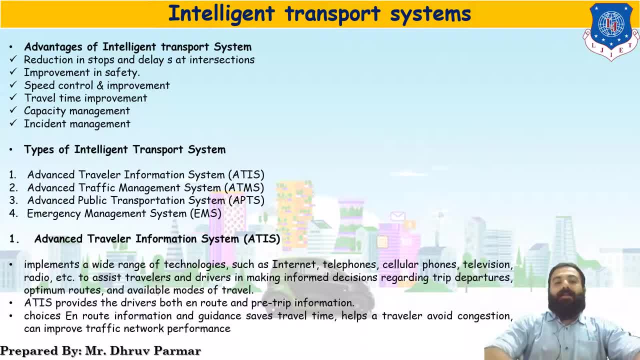 intersection. yeah, you know that intersection we are round about. you can wait. are you almost wait 1 minute or 2 minute? so that time will be reduced by this method, and by this method you improve the safety. then, third one, that speed can be controlled or speed can be improved. 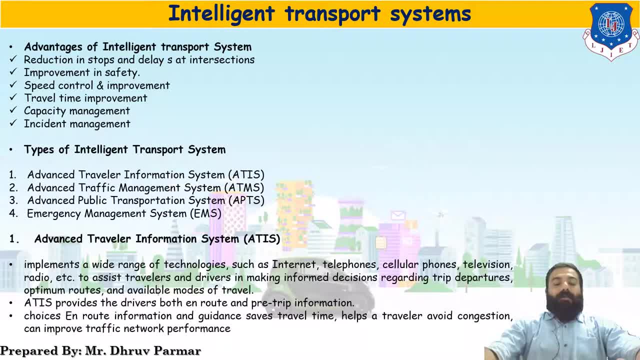 by this ITS. the next one, that travel time, which improved by this method, then capacity management- means the road capacity is- will be increased by the ITS incident management. these are the advantages of ITS. there are types of intelligent transport system. there are 4 types of ITS. first one: advanced travel information, advanced traffic management system. 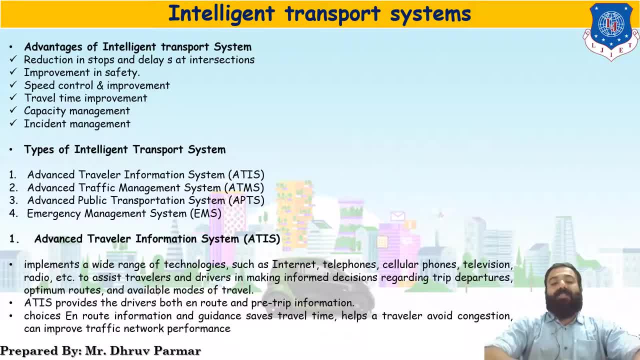 third, one advanced public transportation system. fourth one: emergency management system. clear. so then we will discuss in detail. So first one advanced travel information system, that called ATIS. ATIS means implement a wide range of technology such as internet, telephone, cellular television, radio, to assist travelers. 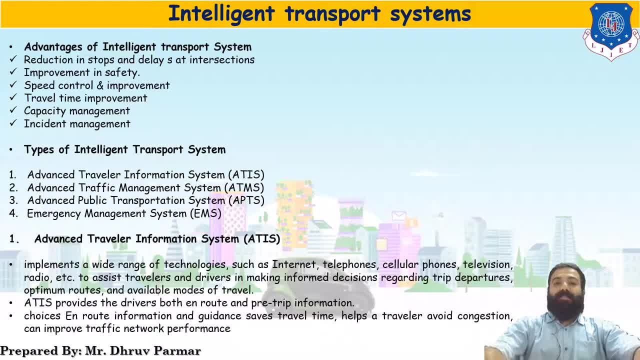 and drivers in making informed decision regarding trip departures and optimum routes and available borders of travel. so you know that by cellular phone, by internet, by maps, you can inform and get the direction of your destination clear, or you can easily predict the weather by this system, so that called advanced traveler information system clear. so ATIS provide the 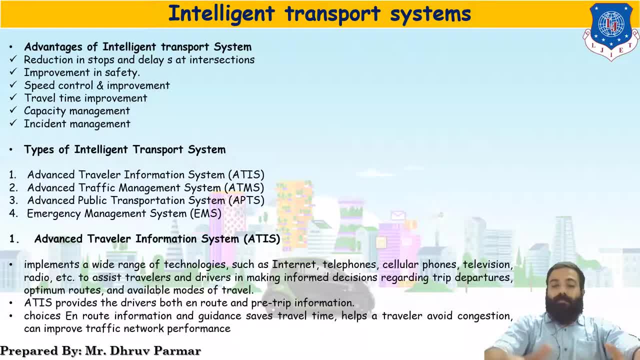 drivers, both android and pre-trip information means report the trip information you get by advanced traveler information system. So that's it. Thank you That en route information and guidance by this system you can save travel time or you can reduce the travel time clear and it helps to avoid traffic congestion because you already. 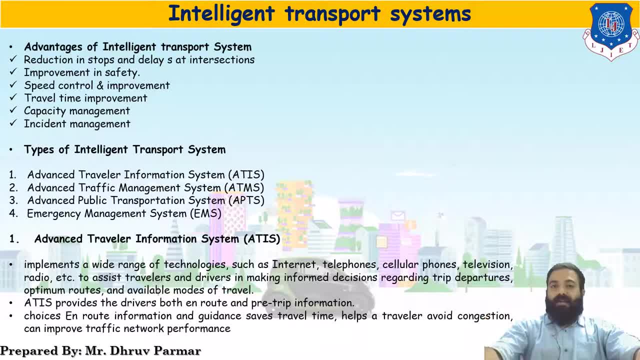 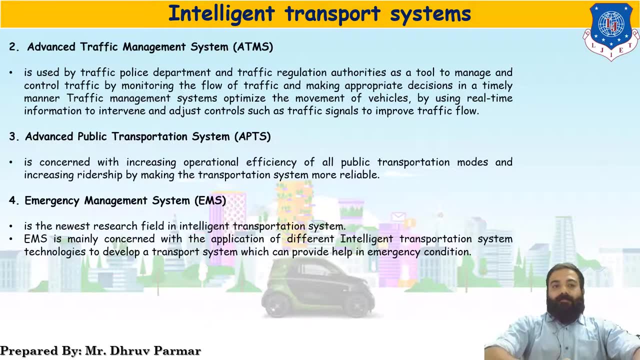 aware about that. that place have a more traffic so you can choose alternate route to reach your destination. clear. Second one, KTMS means advanced traffic management system. clear. so this system is used by police department or traffic regulation authority. for what? as a tool to manage the traffic control by monitoring. 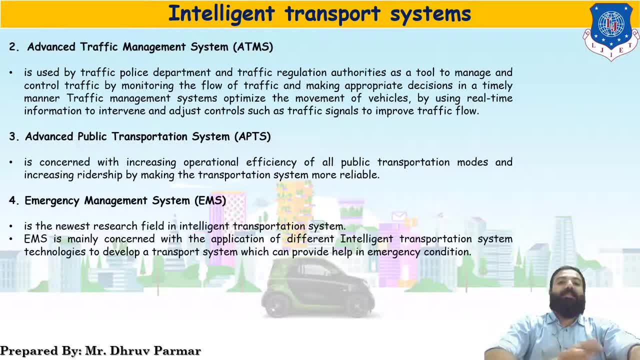 the flow traffic and making appropriate decision on timely manner. clear, so this is a real time information matter. so it is used by police department and traffic regulation authority. clear, it is one type of tool which manage or control the traffic by monitoring the flow of traffic. then third one, APTS means advanced public transportation. clear, so it is concerned. 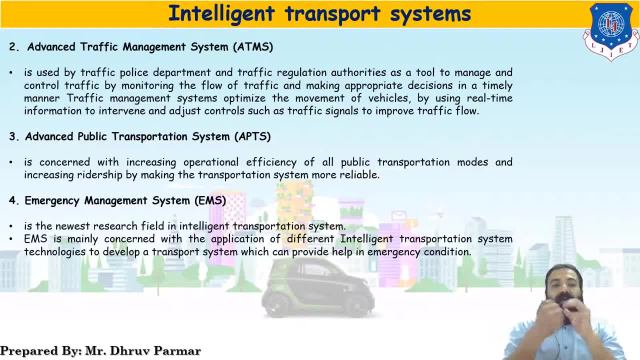 with operational efficiency of public transportation mode, like BRTS, ANTS, SQS, RTS, that all these include in the APTS clear. so this increasing ridership by making transportation system more reliable. then, fourth one, emergency management system: clear. so it is the one type of newest research field in ITS: clear. it is concerned with the applications. 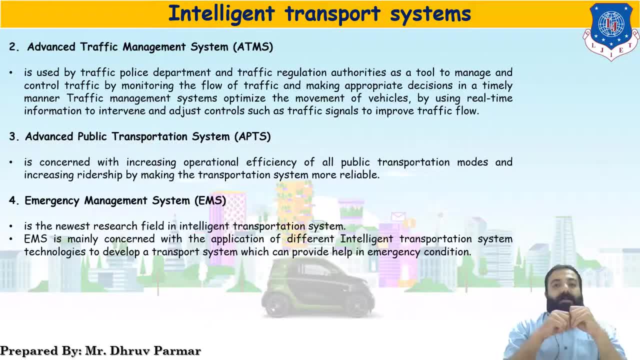 of different ITS technology to develop transportation system. The fourth system, which can provide emergency condition, as per the name, you know that. what is the meaning? means it is used for emergencies, condition clear, like when disaster occur. so that time this system are used clear, but it is the newest method and there are some research. 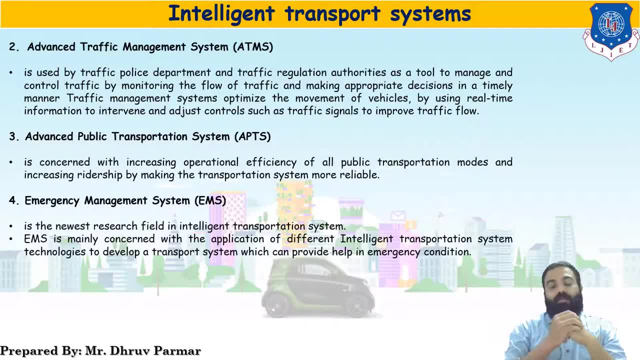 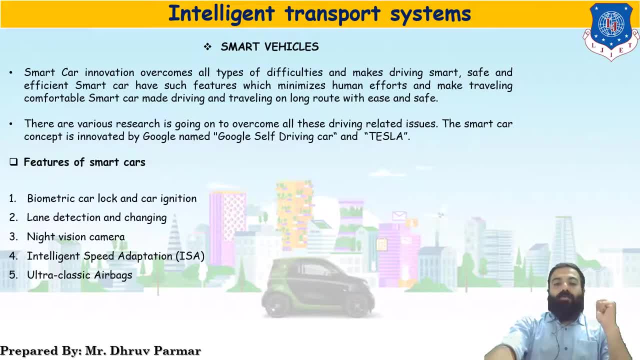 is going on. There are four types of ITS. The next one, smart vehicles. you already about that smart vehicle. what is the meaning of smart vehicles? clear? so that means by the smart vehicle you can overcome different types of difficulties like accident, traffic congestion. then people can do accident by some silly. 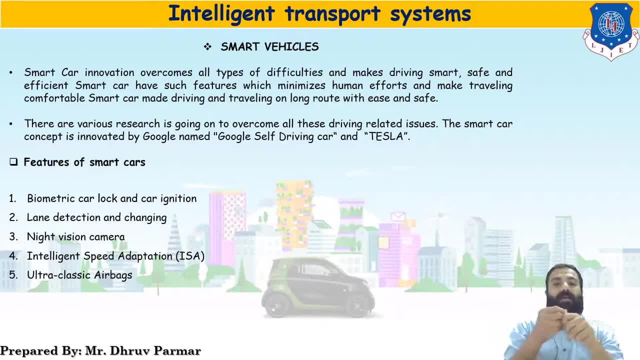 mistakes, so that all thing which is overcome by the smart vehicle clear. so this smart vehicles makes driving smart, safe and efficient clear. so smart vehicle have a different types of features, different types of features which minimize human efforts, make travelling, make travelling comfortable like a Tesla clear. so in Tesla you know that there are auto parts. 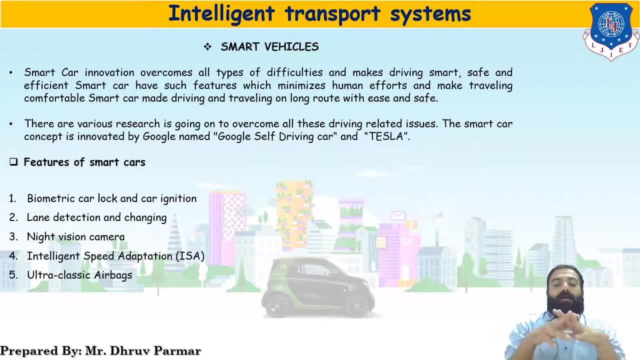 autopilot so you can easily reach, or you can get comfort in this car. clear, so you can easily travel on long route with comfort and safe. there are lots of type of research are going on to overcome this driving related issue. Clear. so, like a Tesla, I am able self-driving car, which are the newest concept, done. so what. 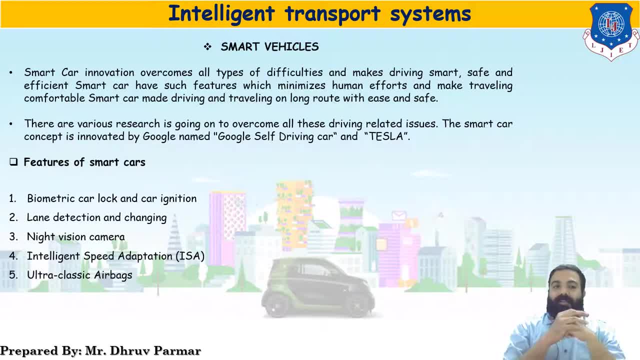 are the features of smart car or smart vehicles. so first one, biometric car lock and car ignitions, then second one, land detection and changing night vision camera. then, fourth one, intelligence speed adaptations. fourth, fifth one, ultra classic airbags. there are five features which are included in smart vehicles. 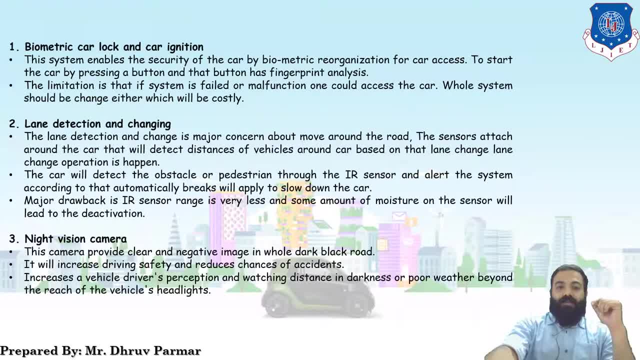 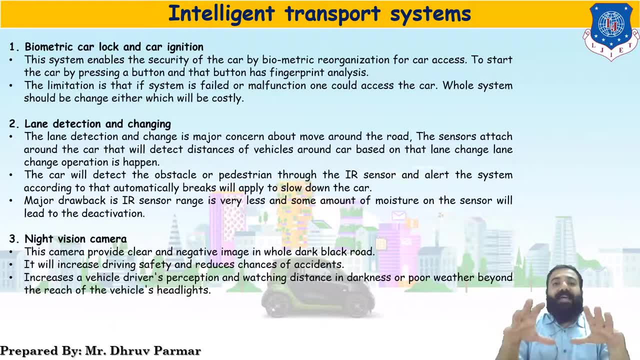 You can discuss in briefly. so first one: biometric car lock and car ignitions. so you know that different types of car, the handle of this car, have a biometric sensor. so you can open a car without key by your finger, sensor clear or you can access and you can start the car. 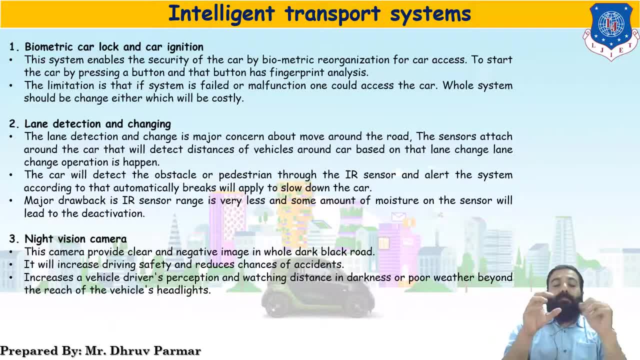 by pressing the button. clear, Because button has a function: Fingerprint analysis or fingerprint sensing. so what are the limitations of this system? clear, so this system is failed or malfunctions, one can access, one could access the car. clear, so that whole system should be changed either, which will be costly. clear, like if you sold. 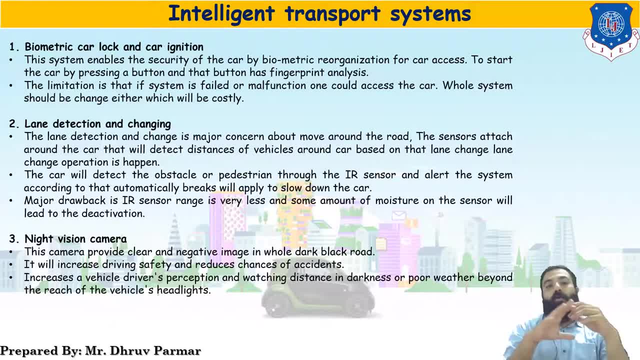 the car to someone, so that whole system should be changed, which is very costly. then second one, land detection. You know that there are many people who change the lap without indicating the sideline, so this is one of the biggest issue in our India. clear so that sensor attached which around 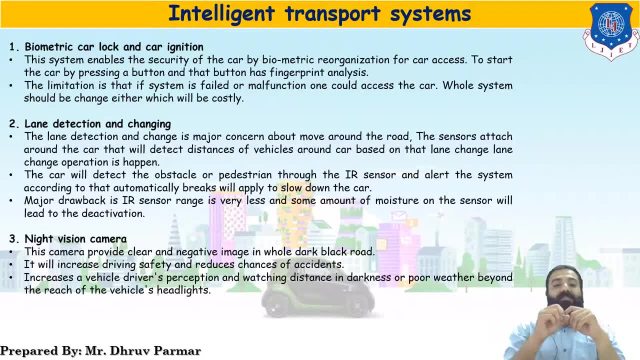 the car that will detect distance of vehicle around the car based on lane change, and lane change operation is happening clear. so there are sensor which are attached to the car and around the car which detect the distance about or distance between cars and you can easily change the lane. then the car will detect the obstacle or pedestrian through the IR. 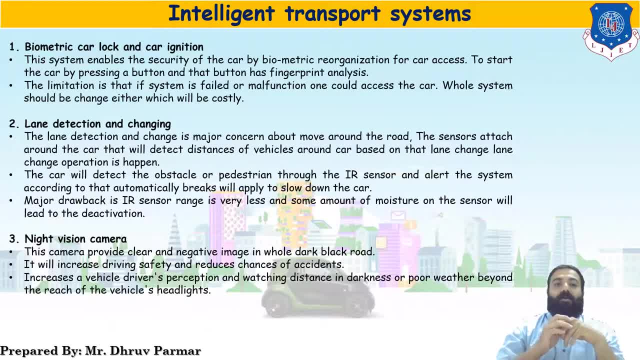 sensors and alert the system according to the automatically brakes will apply to slow down the car. clear, like when you are driving a car on a road so that obstacles or some peoples are working on pedestrians and you can not see or you can not aware. otherwise, you operate some your cell phone so that IR sensor which easily detect and alert the system. 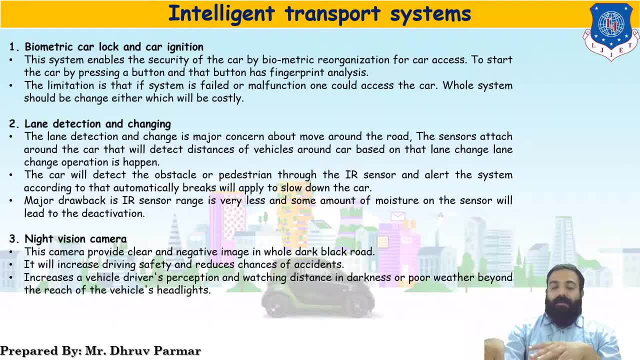 and apply automatically, brake and slow down the your vehicle or your car. so one of the limitations of IR sensor: that range is very less clear, clear like one meter, two meter- and that some amount of moisture on the sensor will lead to the deactivation. then, third, one night vision camera. so this camera provide clear and negative 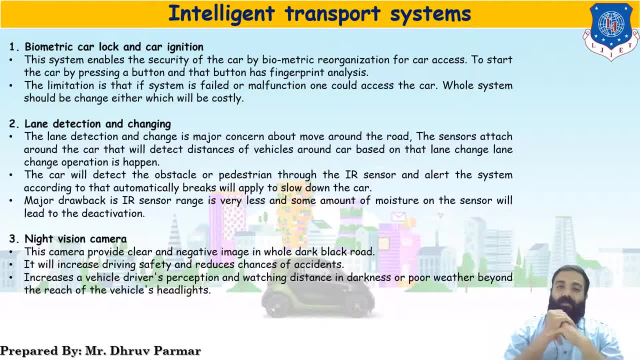 image in the whole dark black area clear. so you know that night vision camera about that, so that provide clear image in night. clear so it will increase driving safety and reduce the chances of accident. you know that there are most of the accident occurs in night due to improper visibility. 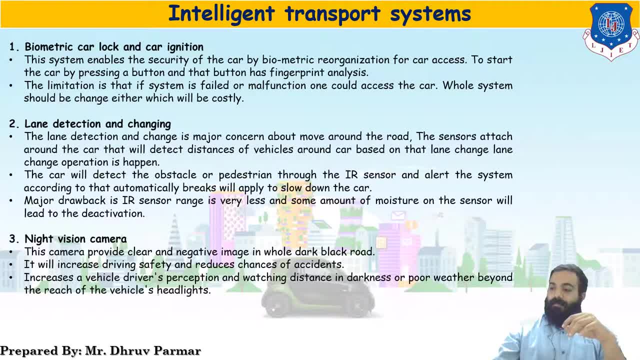 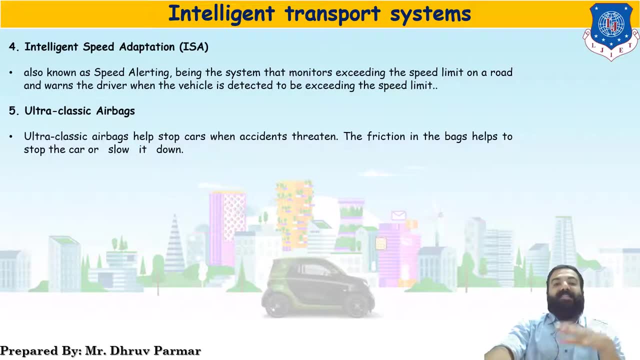 clear, so increase the vehicle driver's perceptions and watching the distance in darkness and where the where the reach of vehicles get clear. so the next one, intelligent speed adaption. so in ISA it is also known as a speed alerting. it means the system monitors exceed the speed limit on a road and warns the driver when 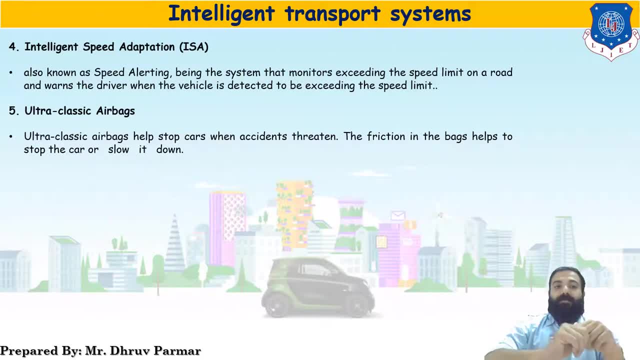 the vehicle is detected or to exceed the speed limit. it means when the vehicle reach over the speed limit, so that system or that sensor which detects the speed limit and warns the driver: you are over speed. then, fifth one, ultra classic airbags: clear. so these right airbags helps. 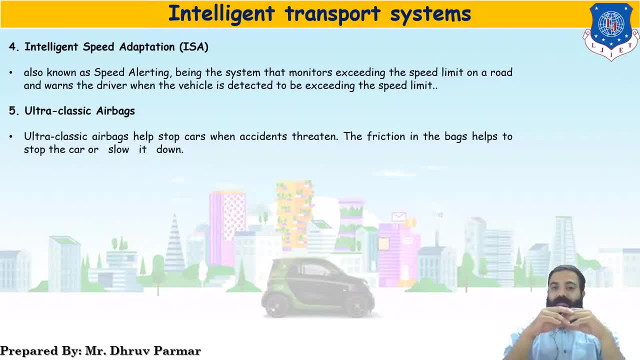 stop the car when accident affect. you know that about different types of airbags. the frictions in the bags help to stop the car or slow it down. this is a ultrasonic, ultra classic airbags. so there are five features which are included in smart maker. so next one: there are different. 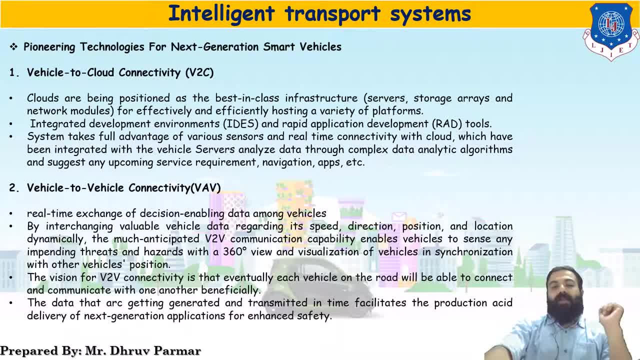 type of technology for next generation, for smart maker. so that will be discussed in next lecture.